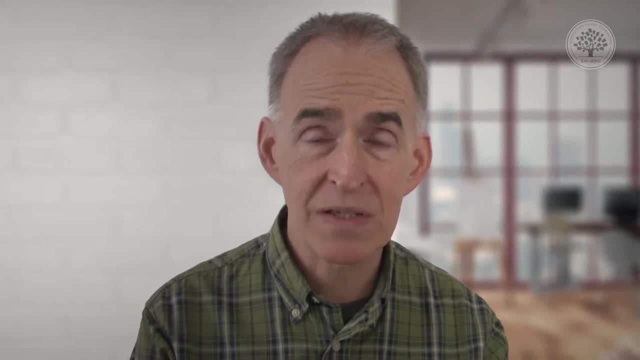 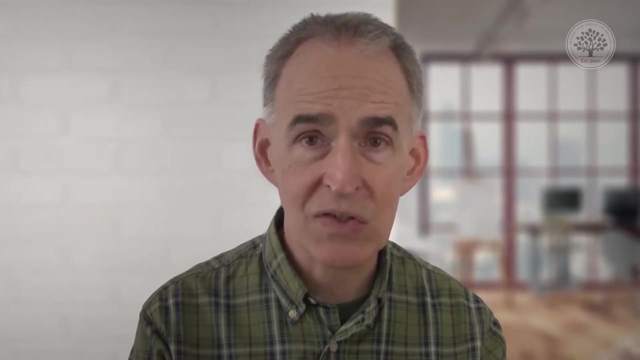 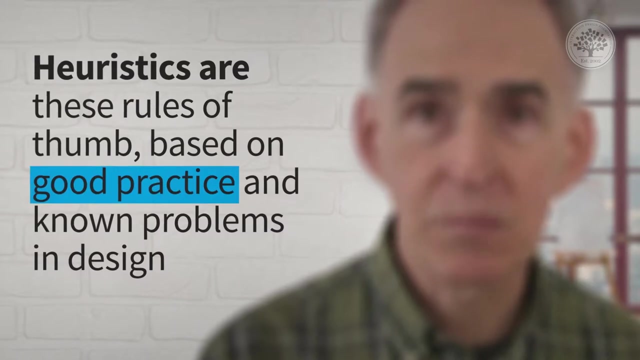 would look like, because as you're doing evaluations and as the industry changes on a regular basis, then you have to appreciate whether or not the solutions you're seeing actually conform to the guidelines in front of you: Heuristics- are these rules of thumb based on good practice and known? 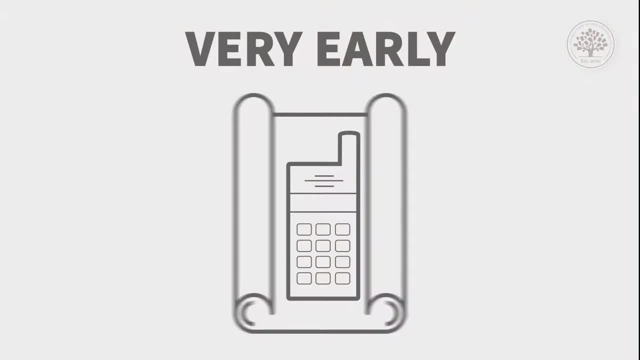 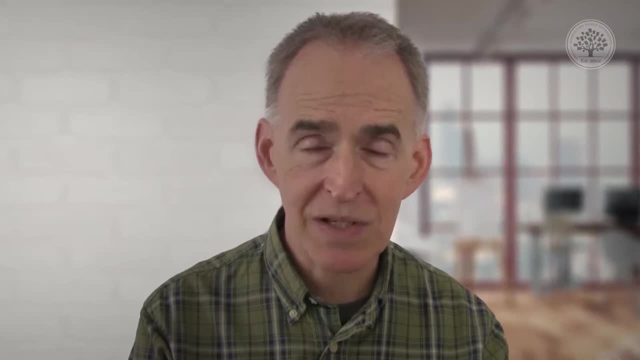 problems in design and they can be used from the very early design through to finished solutions, and you can even do expert or heuristic evaluations on just sketches. if you're doing evaluations, If that would be helpful, It probably is more sensible a little bit later in the process, but 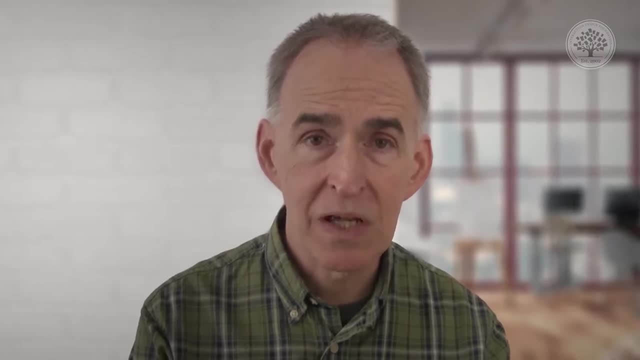 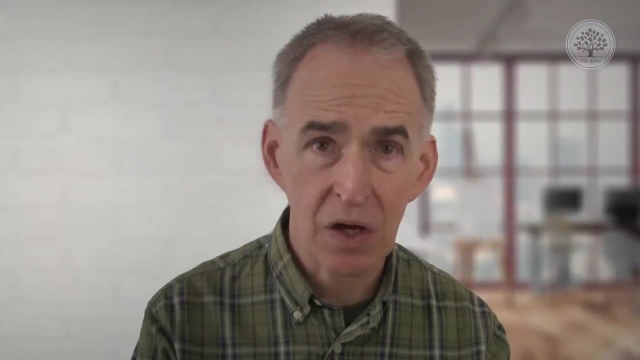 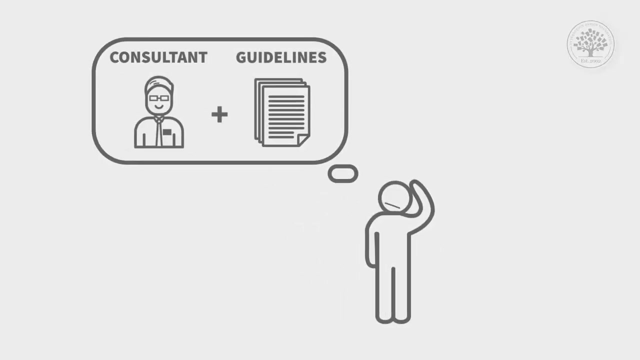 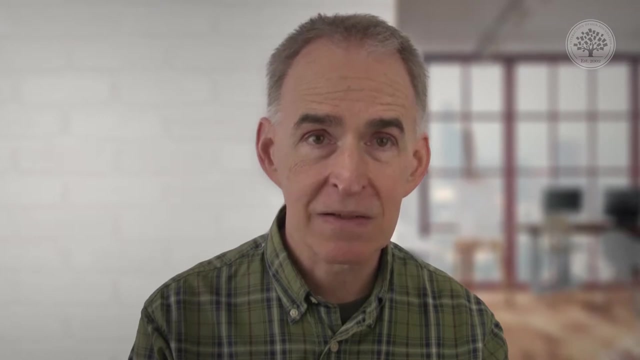 certainly there's no impediment to looking at maybe, the general layout of screens and saying, well, this screen is quite possibly overly complicated for the problem in hand and the hiring in a consultant for one or two days is actually very much cheaper than conducting usability. You can do usability evaluations, but immediately following you'll notice that I mentioned that it's 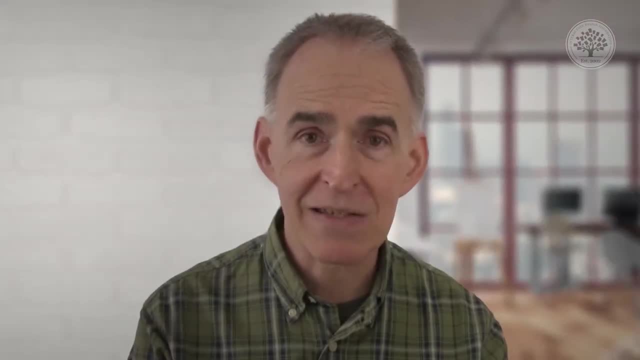 not as effective as testing with real users, and that is certainly the case. However, if you had a lot of novel designs and you wanted to get some idea about whether they were going to be effective, then inviting people in who actually do usability testing, who are experts in. 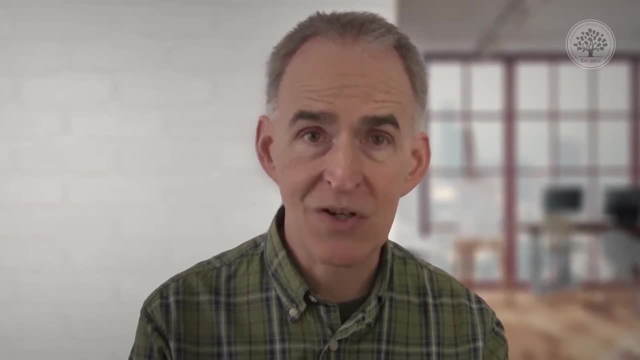 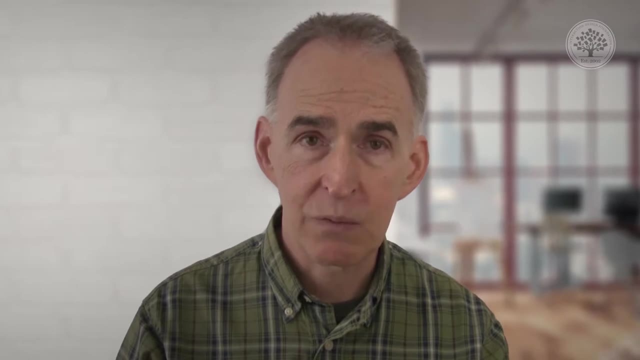 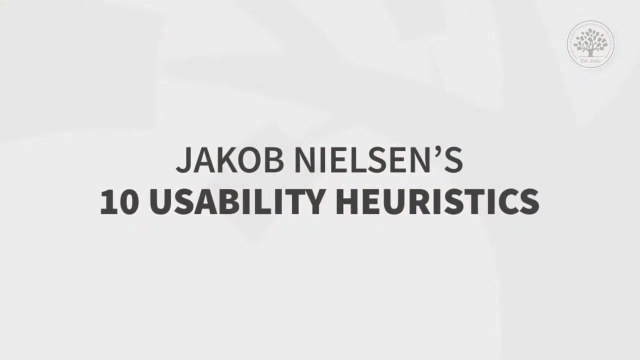 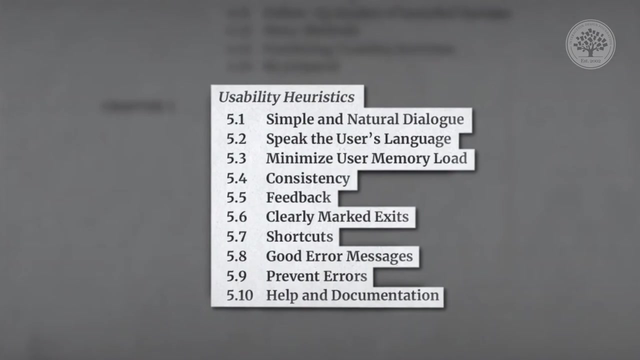 the field will get you a lot of feedback without nearly so much cost as a lot of usability testing, which is a lot of work. It can get quite expensive just because of having to recruit, reward hire facilities and so on. Jacob Nielsen published his book on user interface engineering back in the early 1990s, and these are 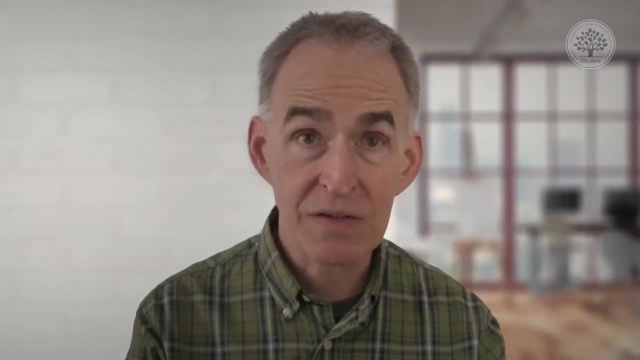 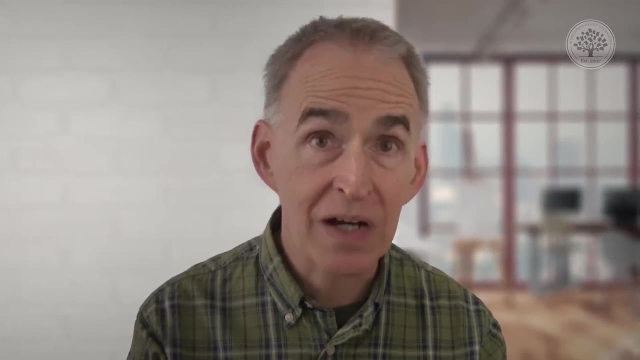 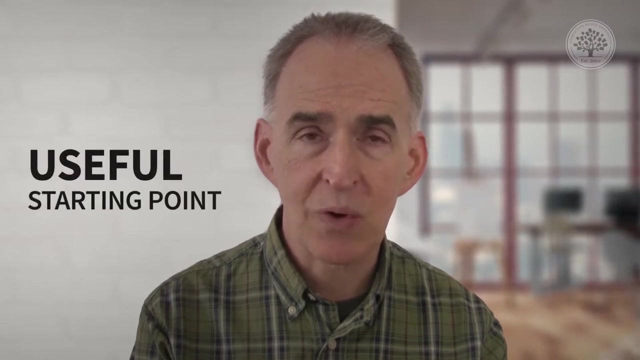 his 10 basic UI user interface heuristics and they haven't really changed, Although when we actually go out to do something like benchmarking we have a very much more detailed set of heuristic. but these are a useful starting point and they're talking about fairly 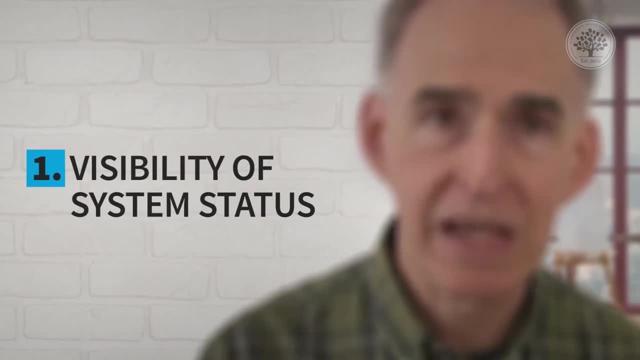 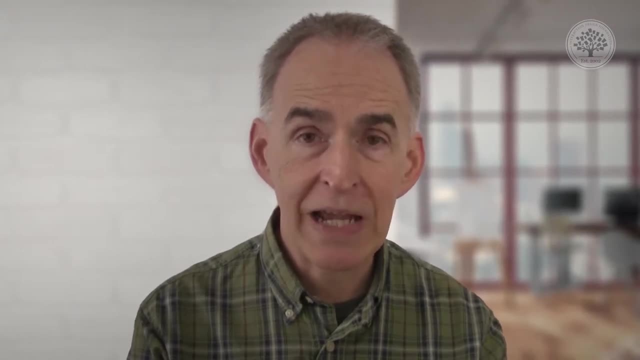 generic concepts like visibility of system status and making sure that people understand where they are in the process- and that, of course, is a good thing, no matter what you're doing- and detailed design does actually flow out of that, for example, letting people know that they've got things in. 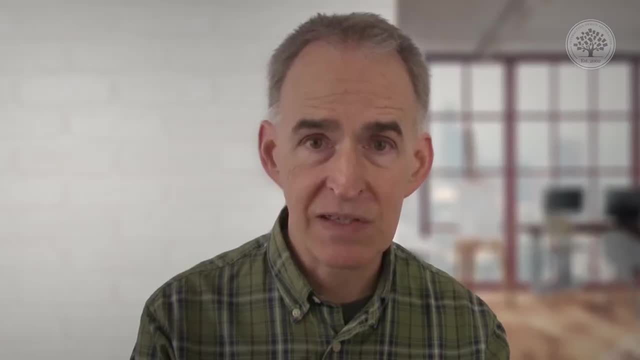 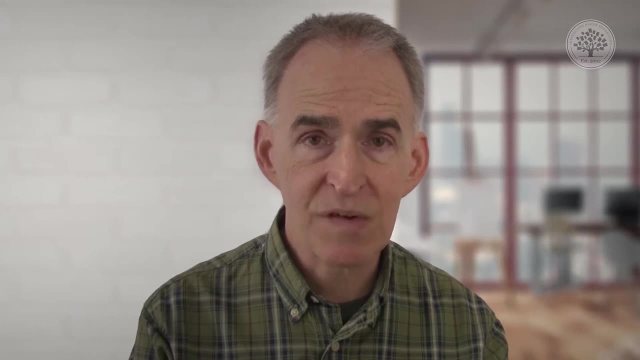 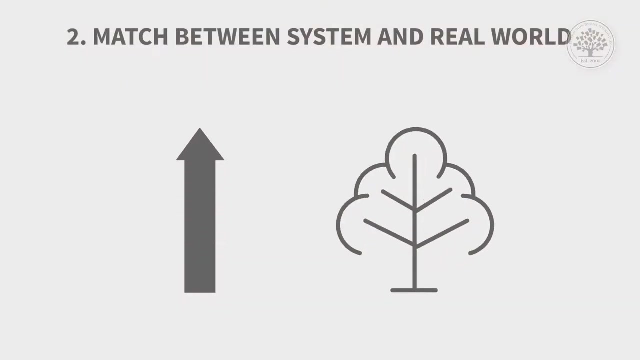 their shopping basket. That is an example of the visibility of system status Match between the system and the real world and that's something I've already alluded to when I was referring to terminology. The mapping sometimes is also physical. You're talking about the natural tendency for increasing the quantity of something. it tends to be up. 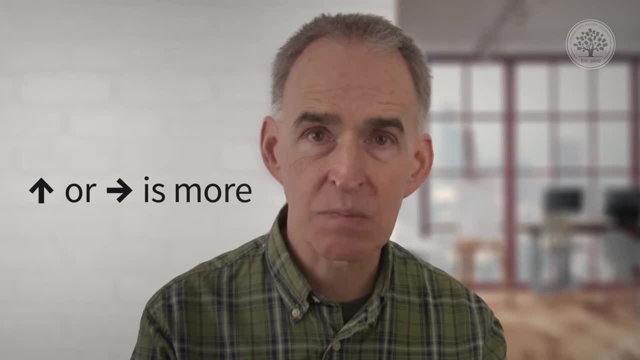 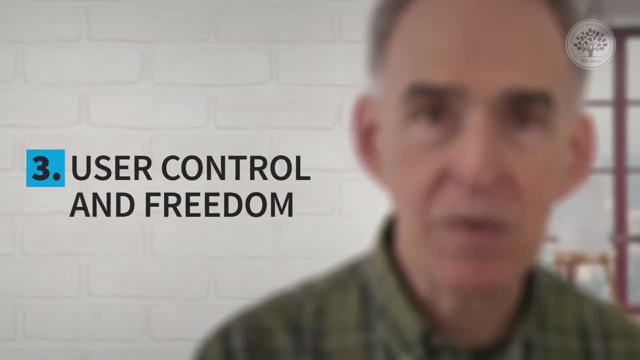 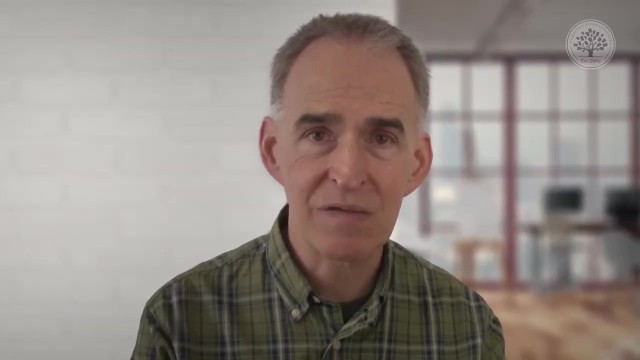 So if you've got a slider, then up or to the right is more and down or to the left is less, and that's just what we call natural mapping. Our user control and freedom are being flexible, allowing people to go back and fix things. Bear in mind that when user interface design was relatively new on the sort of the large scale back in the 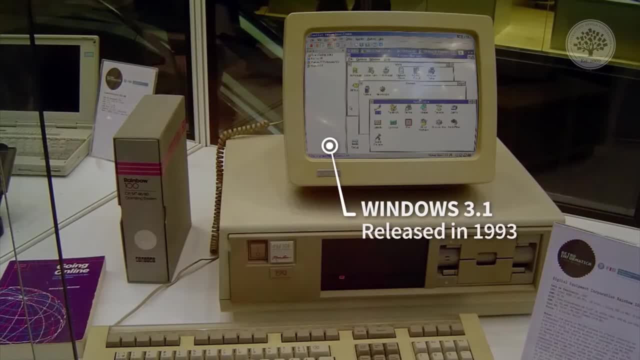 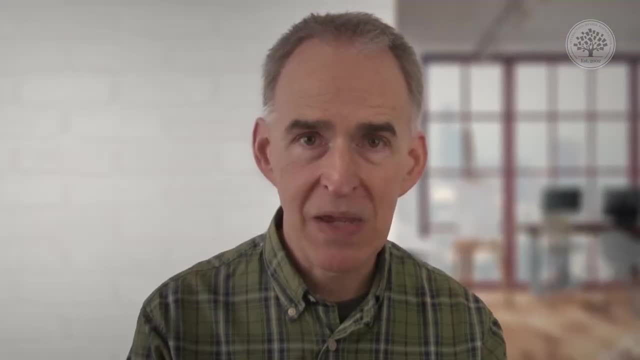 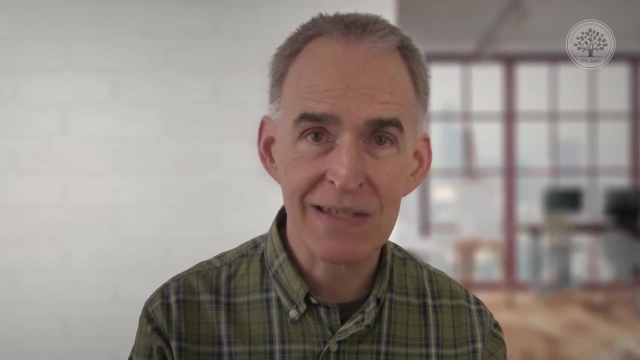 1990s, when Windows 3.1, which was kind of the very first successful version of Windows, and of course World Wide Web came around about the same time. it was uncommon. it was very unusual to have undo functions. If you made a mistake and you needed to fix it, then you had to fix it yourself. 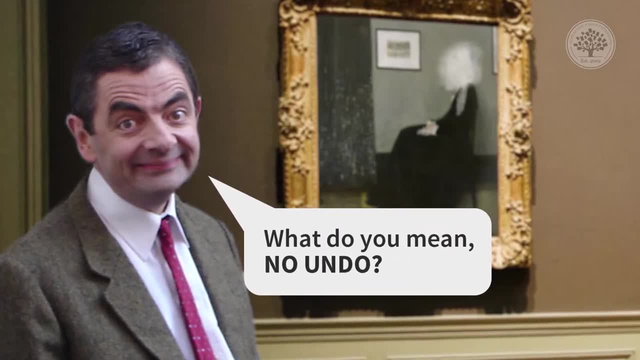 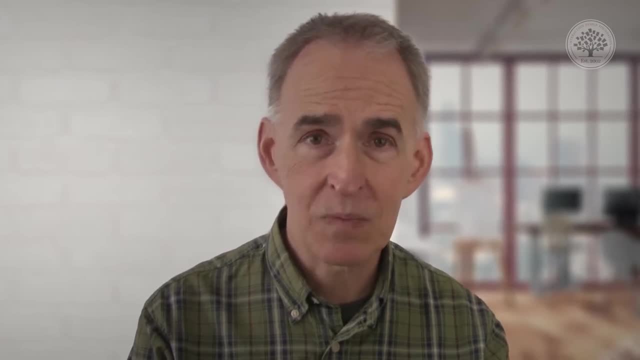 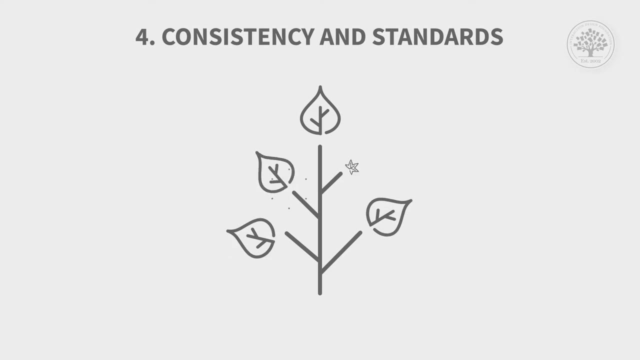 There was no control. Control, said, or any kind of undo facility was something that you had to do, And we take that for granted now, But it was not the case in the early days. Consistency and standards: users should not have to wonder whether different words, situations or actions mean the. 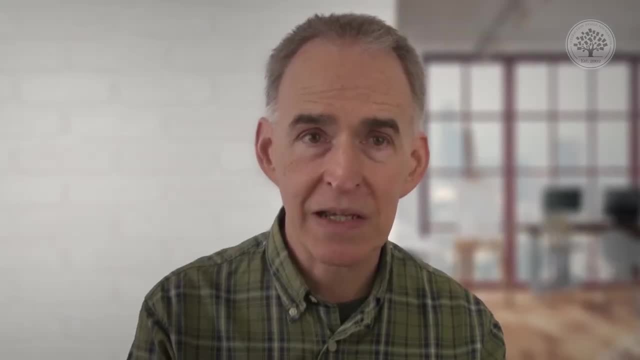 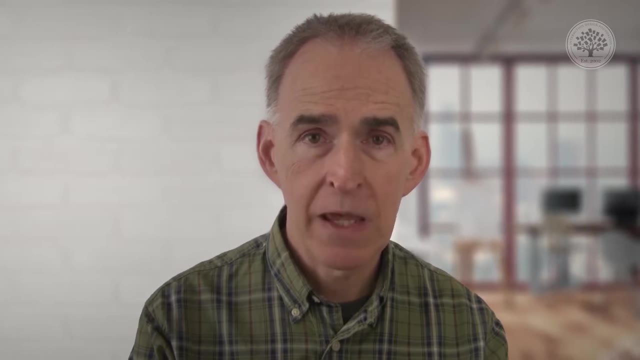 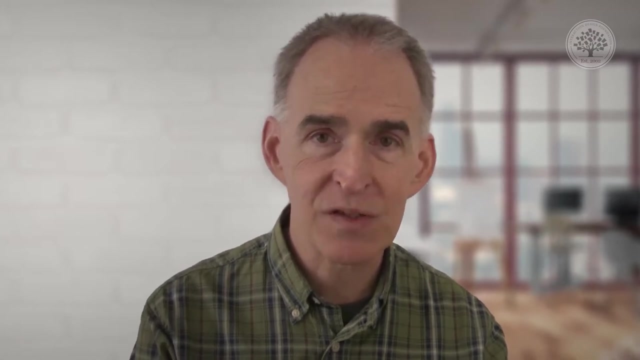 same thing And this continues to be a problem in some areas, certainly on intranets within large organizations, You would find that one department had its own set of visual guidelines, With its own visual language, which was totally different to the next department. and if you 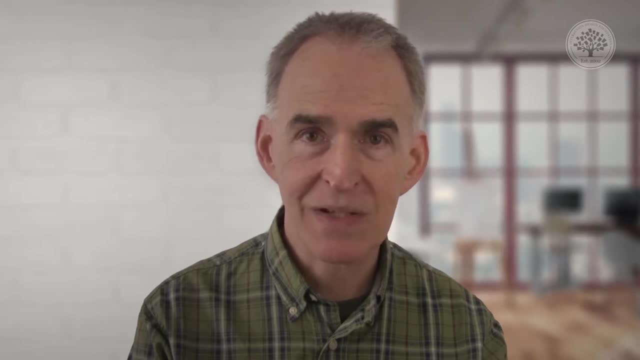 were unlucky enough to have to move between those departments on the intranet, then you were in a bit of trouble. It doesn't happen so much these days with the web e-commerce, for example. people do try very hard to make sure that users are going to have a fairly painless experience, and so 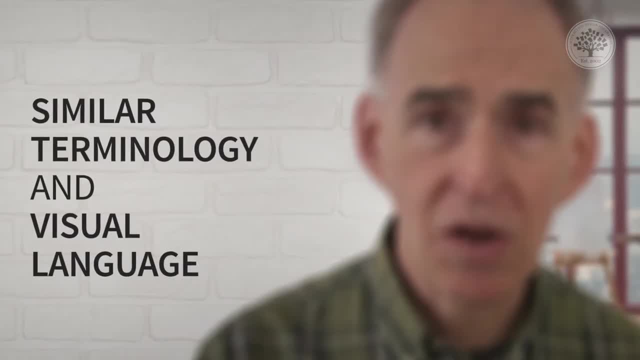 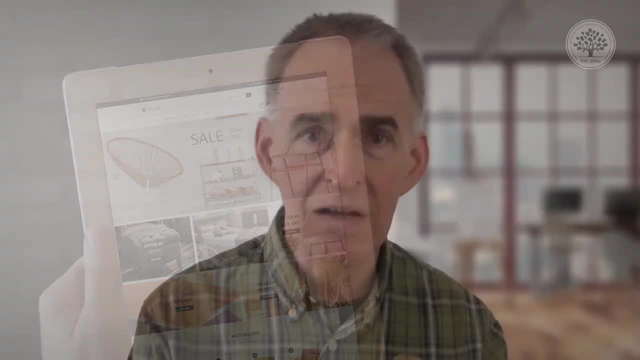 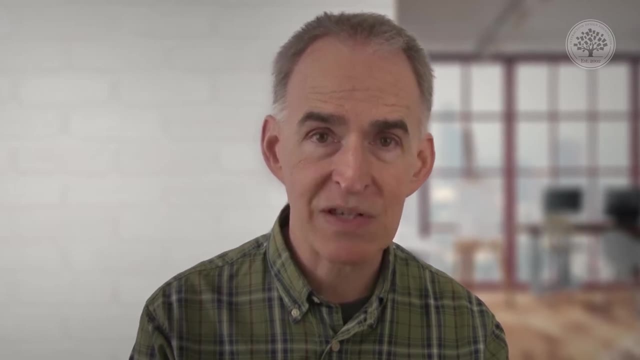 we do tend to see things laid out with very similar terminology and visual language between totally different E-commerce sites and, to be honest, there Amazon, because they are so large and popular- has been something of a yardstick Most people when they're asking for advice on how to do something in e-commerce. I would 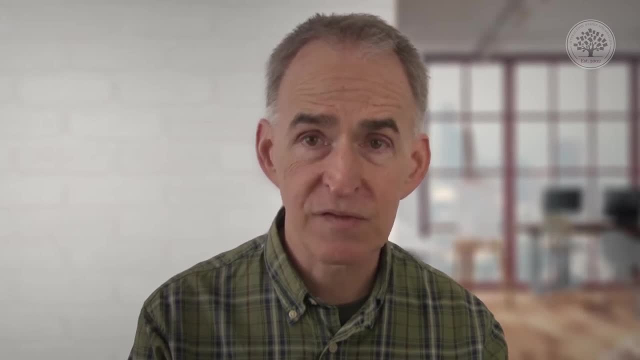 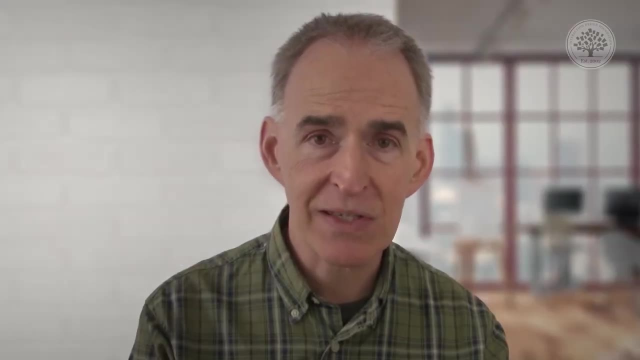 refer them to the Amazon site, and usually for a very good reason. Error prevention is much more successful than dealing with errors. Certainly, if you're having to discard data or if you reject data because users did not understand how you wanted it formatted, You should not. 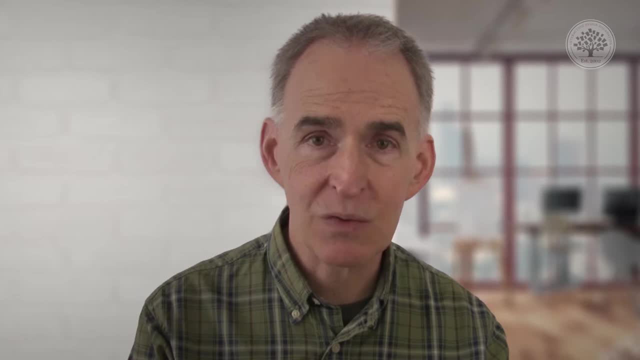 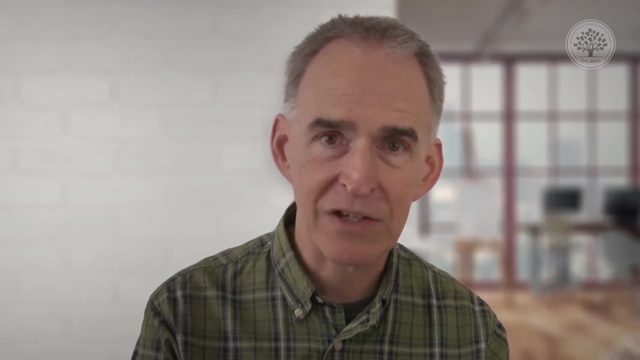 I insist that people punctuate things exactly the way you need them. You can do whatever you like with the punctuation once you've got the basic data from them. If you want the phone numbers without punctuation, then take the punctuation out of the phone number after you've got it. 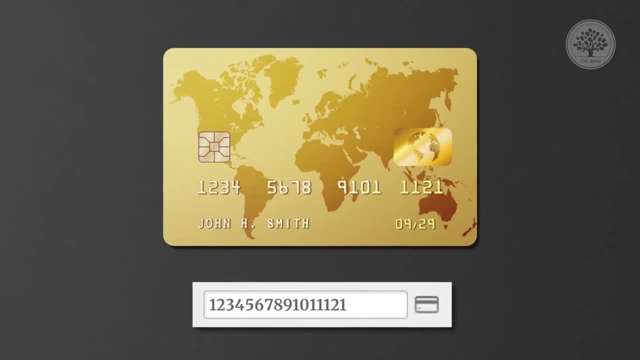 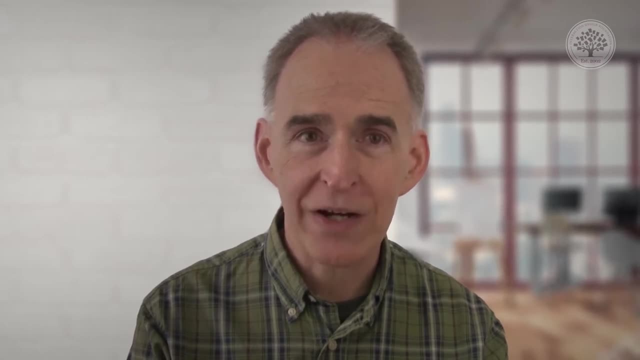 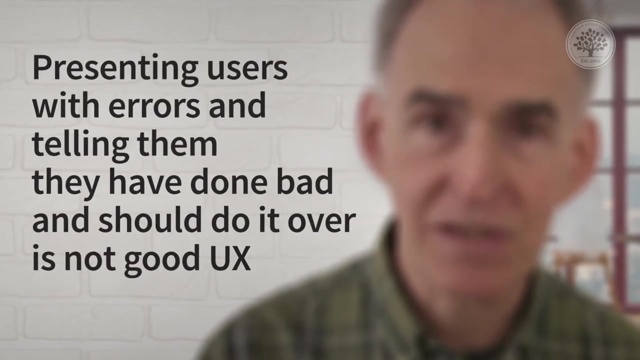 If you don't like the spaces in the credit card numbers, then take the spaces out of the credit card numbers. So that isn't something that Jacob talks about here, but it is a different form of error prevention and I wholeheartedly recommend it: Presenting users with errors and telling them they've done bad and should do it over. 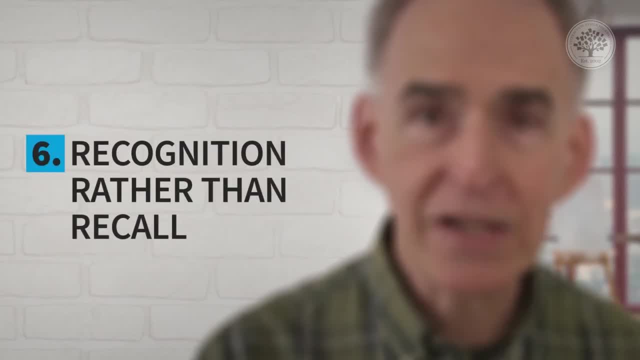 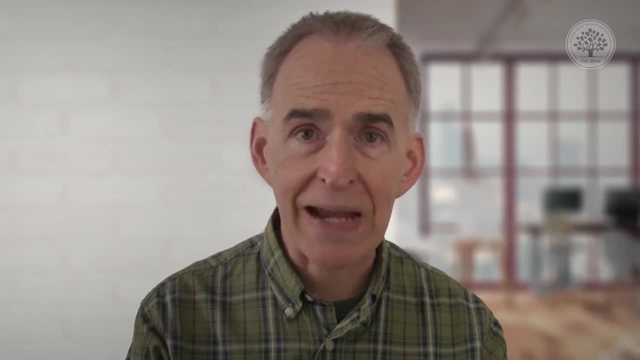 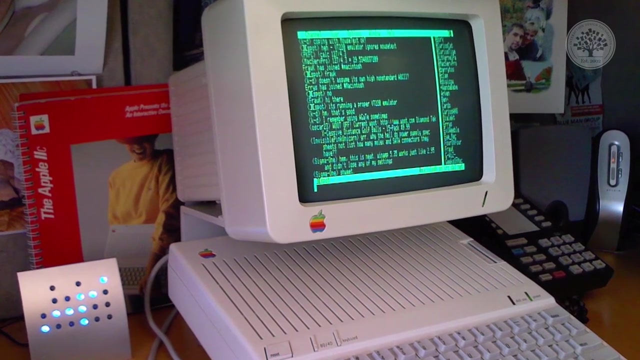 is not good user experience. Recognition rather than recall, and this is the basic premise of all user interfaces these days. That's the way that we've moved. back in the 1970s and 1980s, Most systems were command line based and you had to remember the syntax and spelling of 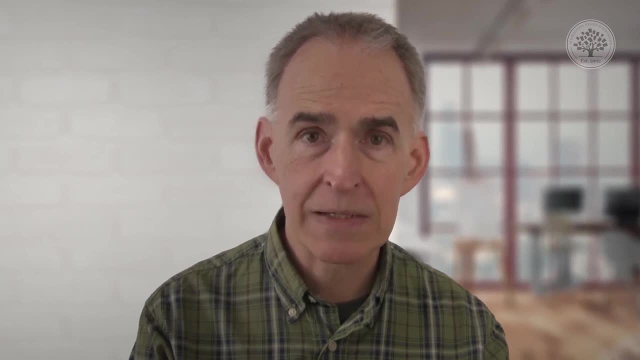 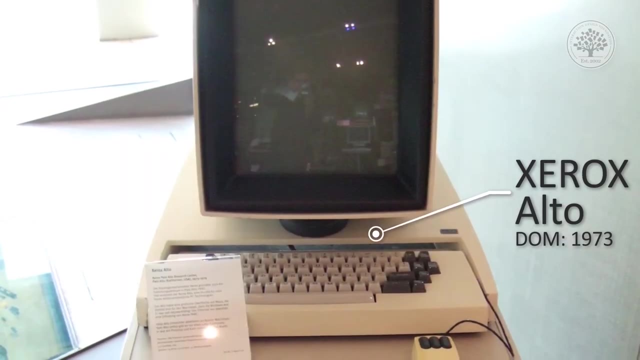 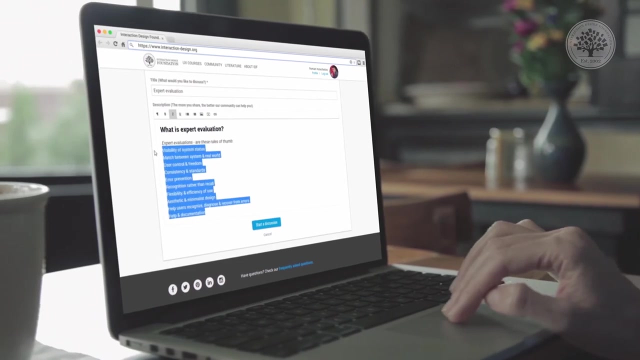 the next command you wanted to enter. and when Windows and the Mac came along, both having stolen their designs from Xerox PARC, then we got what we used to refer to as WYSIWYG. What you see is what you get. We don't talk about that much these days, but it was all about recognition which people 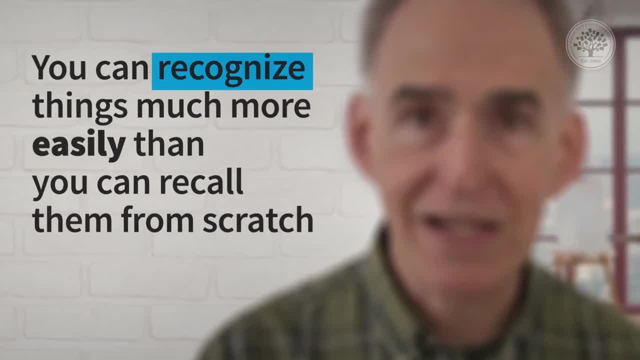 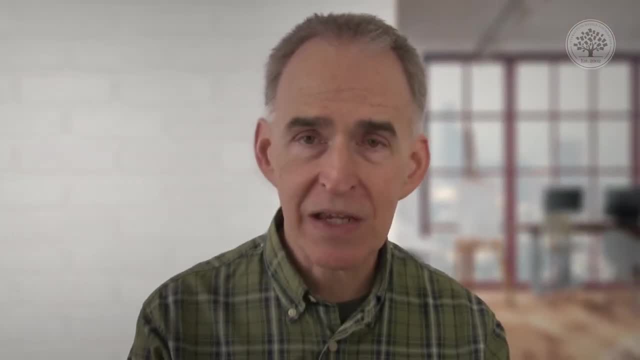 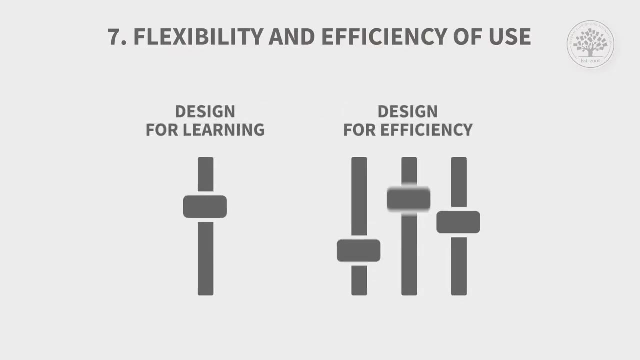 are very much better at than recall. You can recognize things much more easily than you can recall them from scratch. Flexibility and efficiency of use, and usually there is a trade off between what you might call design for learning and design for learning. I'm not going to go into that. 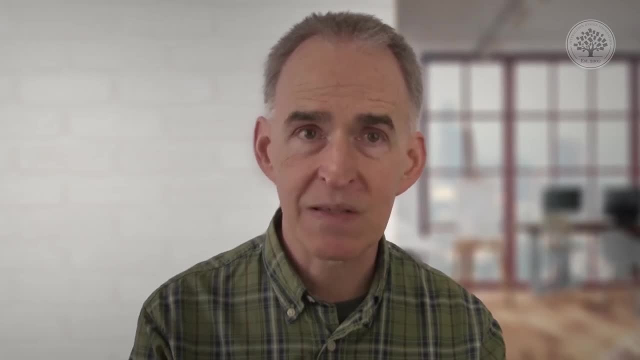 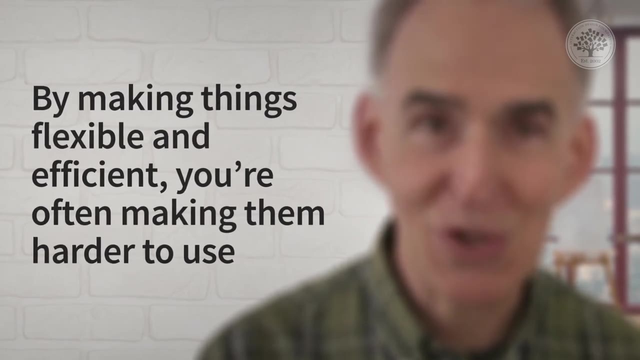 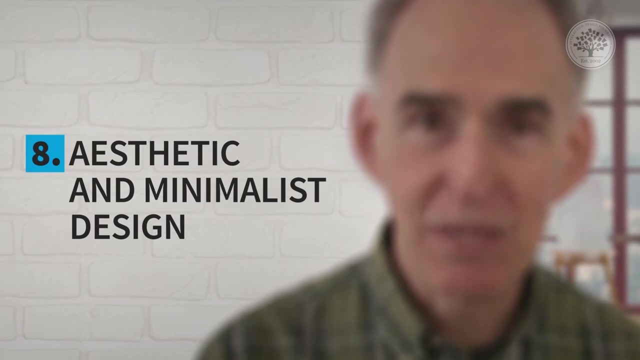 Design for efficiency. That is all tied up with flexibility and efficiency of use. By making things flexible and efficient, you're often making them harder to use, So that's where the tension in the design comes. in Aesthetic and minimalist design, People like websites that look attractive and that they trust from a visual design perspective.